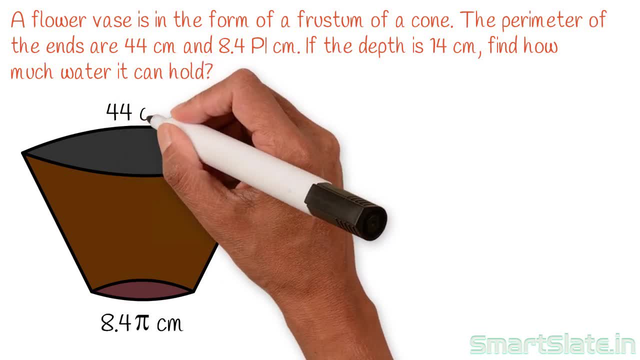 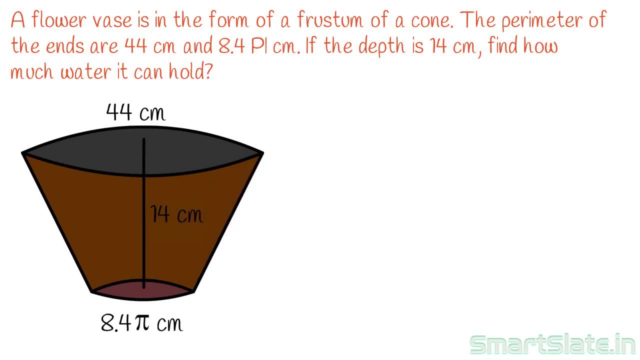 And perimeter of lower base is 44 cm. Depth of this vase is 44 cm. Depth is nothing but the height of this frustum of cone. We are supposed to find how much water it can hold. It means we should find the volume of this vase. 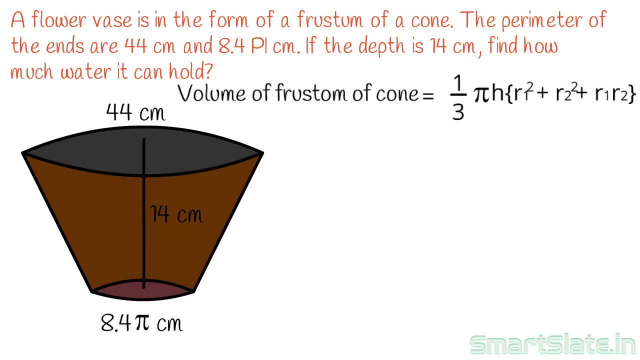 Recall the mathematical formula to find frustum of cone. Volume of frustum of cone is equal to 1 by 3, into pi, into h, in the bracket R1 square plus R2 square. We don't have radii of bases, but we do have perimeters. 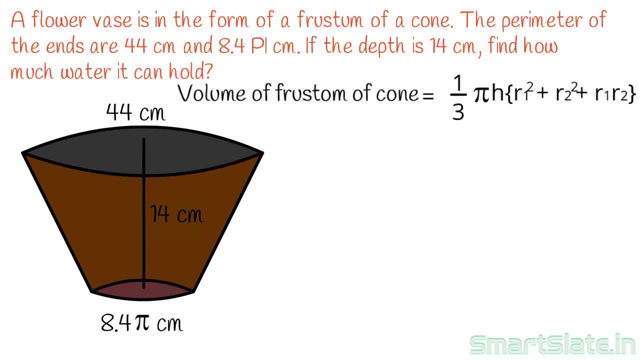 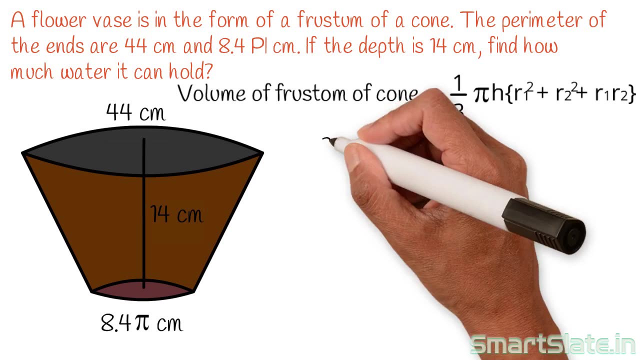 Using the given value of perimeters, let's find the radii. Perimeter of first base is 8.4 pi. Formula to find perimeter is 2 pi R. Let R1 be the radius of first base. Hence 2 pi R1 is equal to 8.4 pi. 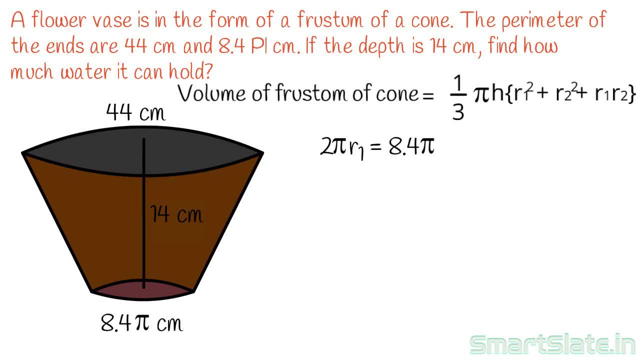 After simplifying this equation, we get R1 equal to 4.2 cm. Let's find second radius: 2 pi R2 is equal to 44.. Hence, R2 is equal to 44 by 2 into pi. R2 is equal to 44 into 7 by 22, into 1 by 2.. 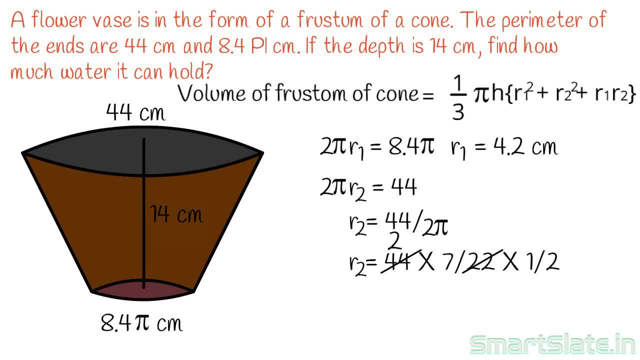 22 divides 44. R2 is equal to 7 by 22 into 1 by 2.. 22 divides 44.. Cancel 2 and 2.. We have value 7.. Hence, R2 is equal to 7 cm. 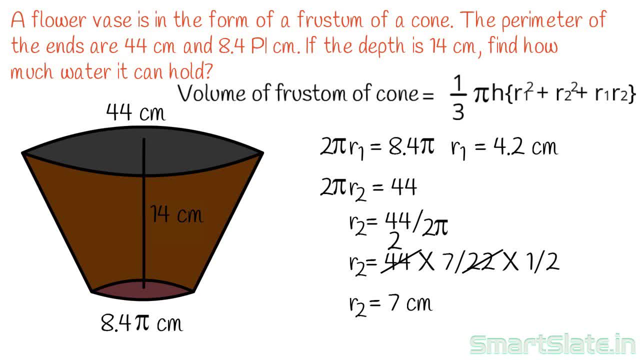 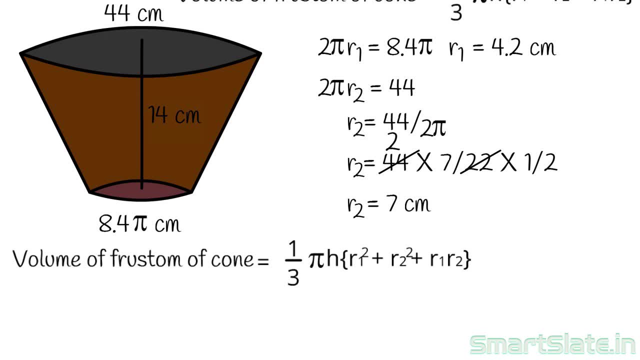 Since now we have value of R1 and R2, we can easily find the volume. Volume of frustum of the cone is equal to 1 by 3 into pi into h in the bracket R1 square plus R2. square plus R1 into R2.. 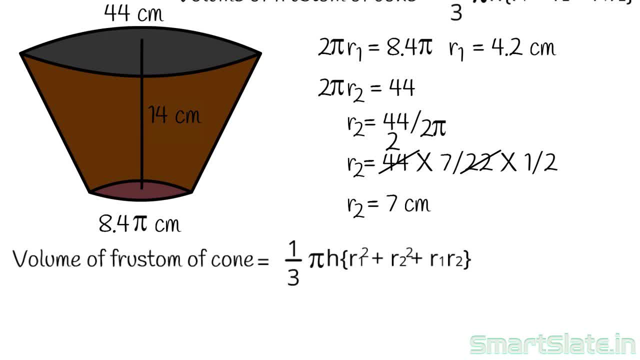 Substitute the value of R1 into R2.. Substitute the value of R1 into R2.. We have value of R1, R2 and height h. It is 1 by 3 into 22 by 7 into 14 in the bracket 7 square plus 4.2 square plus 7 into 4.2 bracket. 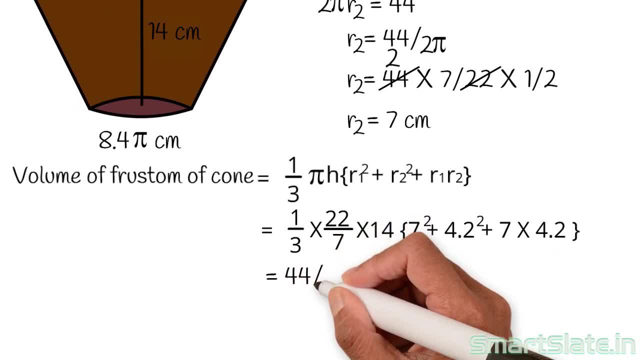 complete. It is 44 by 3 into in the bracket 49 plus 17 plus 64 plus 29.4.. It is 44 by 3 into 96.04.. Addition of 49 plus 17.64 plus 29.4 is 96.04.. 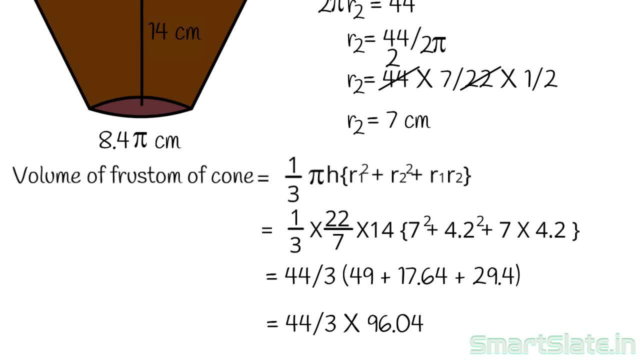 44 by 3 into 96.04 is 1408.58.. Hence volume of frustum is 1408.58 cm3.. Let's solve for volume of frustum. It takes 4 into 1 by 2.. 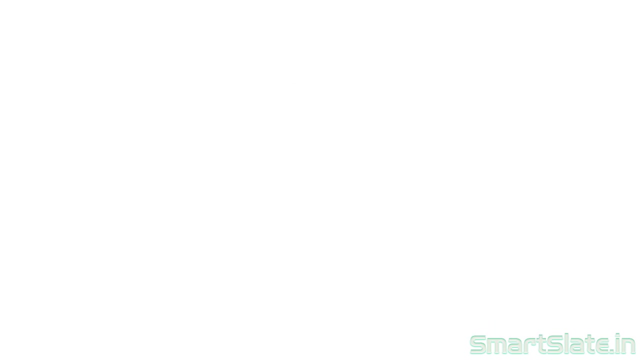 It is 2 by 2.. another problem: A bucket is in the shape of a frustum with the top and bottom circles of radii 15 cm and 10 cm. Its depth is 12 cm. Find its curved surface area and total. 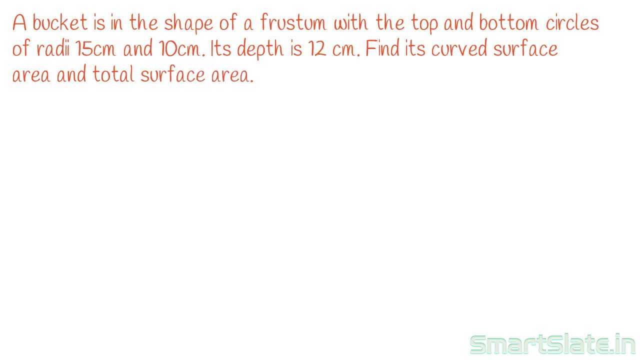 surface area. We have frustum of cone, and question provides data such as radii of top and bottom circles. The depth of the frustum of cone is also given. Using these data, we are supposed to find lateral surface area and total surface area. Let's recall the 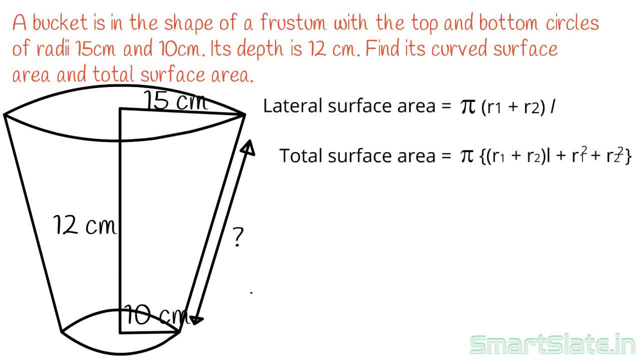 formula to find the same Lateral surface area of frustum of cone is equal to pi in the bracket r1 plus r2, into l plus r1 square plus r2 square. Both of these formula required the value of slant height l. We do have formula to find slant height with given height. It. 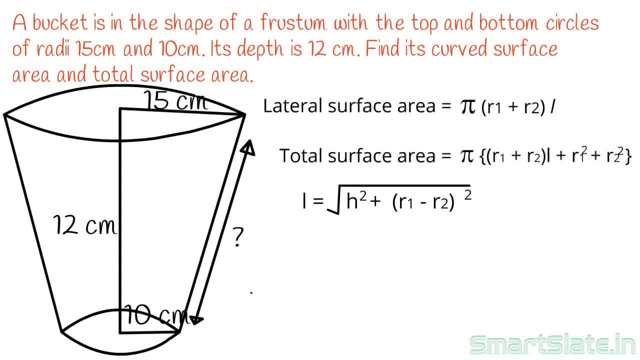 is: l is equal to square root of h square plus r1 minus r2 square. Let's find the slant height and then we can easily find lateral surface area and total surface area. We have the data: h is equal to 12 cm, r1 is equal to 15 cm and r2 is equal to 10 cm. Substitute. 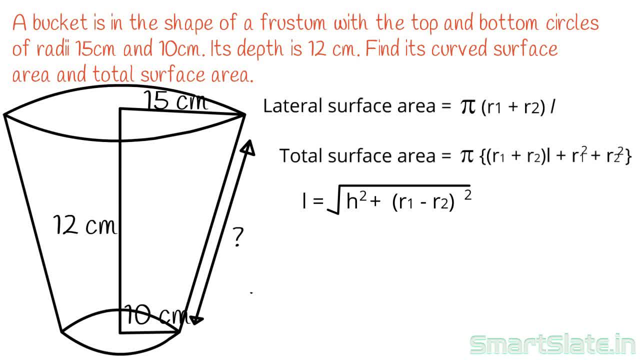 these values into the formula. l is equal to square root of 12 square plus 15 minus 10 square. It is square root of 144.. plus 25.. Because 15 minus 10 is 5 and 5 square is 25.. 144 plus 25 is 169.. It is square root. 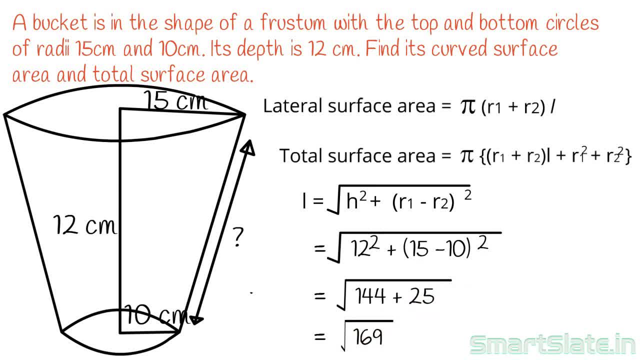 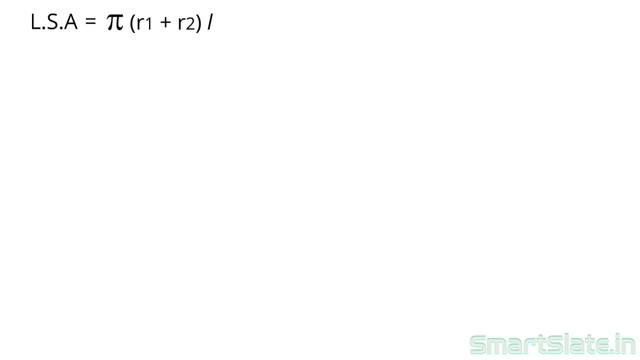 of 169.. Square root of 169 is 13.. Hence L is equal to 13 cm. Now we have the value of slant height. Let's find lateral surface area and total surface area. Lateral surface area is pi in the bracket R1 plus R2 into L. Substitute the values of R1, R2 and L. 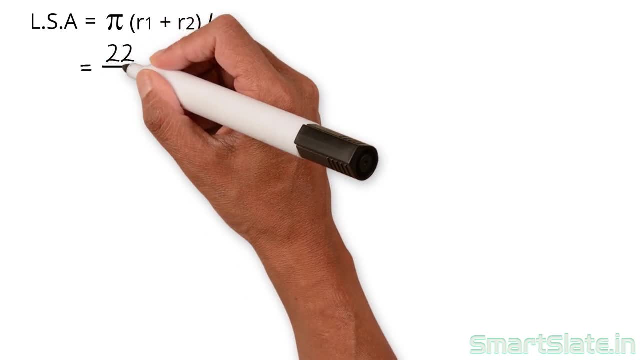 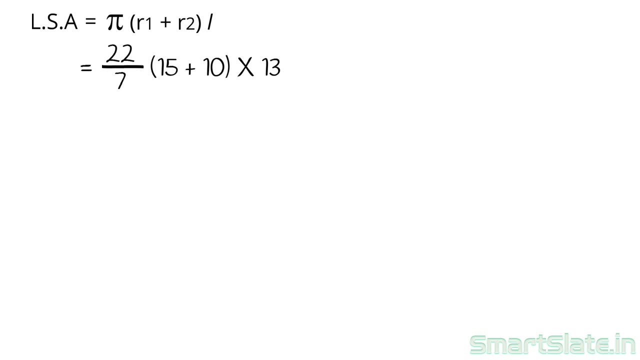 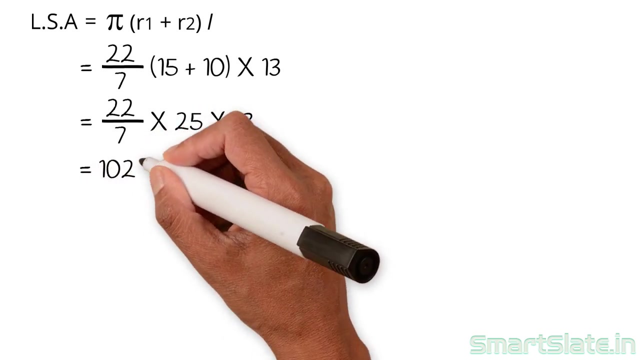 It is 22 by 7 in the bracket 15 plus 10 into 13.. 15 plus 10 is 25.. Hence, it is 22 by 7 into 25.. It is 1021.428.. Hence, lateral surface area is 1021.428 square cm. Let's find the total. 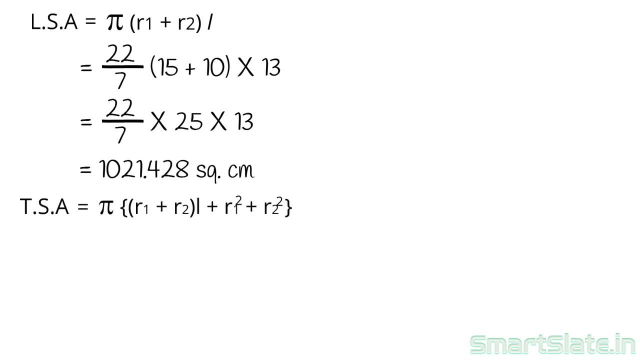 surface area. It is pi in the bracket R1 plus R2 into L plus R1 square plus R2 square. Substitute the values of R1, R2 and L. It is 22 by 7 in the bracket 15 plus 10 into 13.. Hence it. 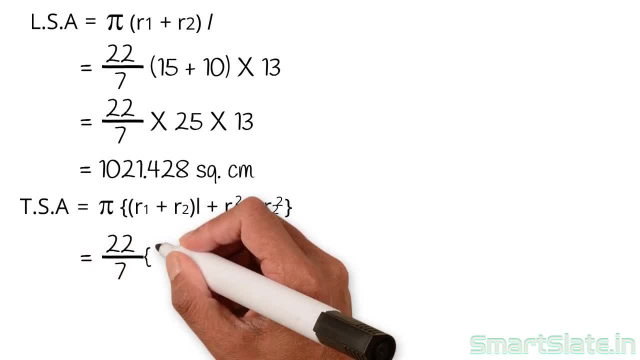 is 22 by 7 into 15 square plus 10 square 15 plus 10 into 15 square plus 10 square 15 plus 10 into 13 is 325.. 15 square is 225.. 10 square is 100.. Hence it is 22 by 7 into. 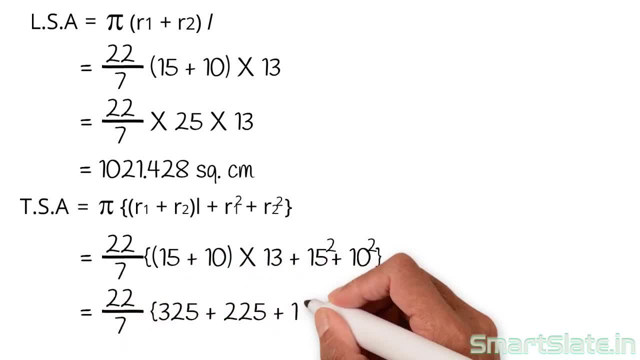 in the bracket 325 plus 225 plus 100.. Addition of these 3 terms is 167.224.. Hence L is equal to 25.. 650.. Hence it is 22 by 7 into 650.. 22 by 7 into 650 is 2042.857.. Hence, total surface. 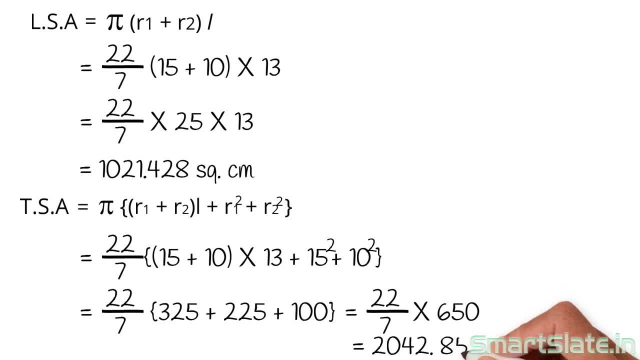 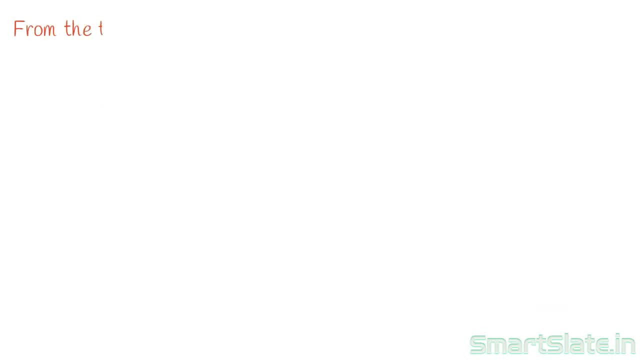 area is 2042.857 square centimeters. Let's solve one more problem. From the top of a cone of a base radius 24 centimeters and height 45 centimeters, a cone of slant height 17 centimeters is cut off. What is the volume of the remaining frustum of the cone? We have cone whose base 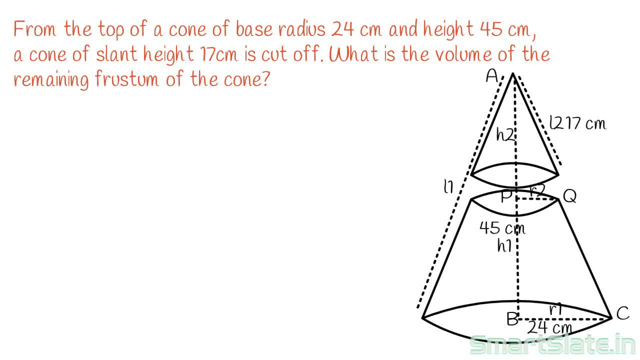 radius is 24 centimeters and height is 45 centimeters. Top portion of the cone, whose slant height is 17 centimeters, is cut off. We are left with frustum of cone. We are supposed to find the volume of this frustum of cone? 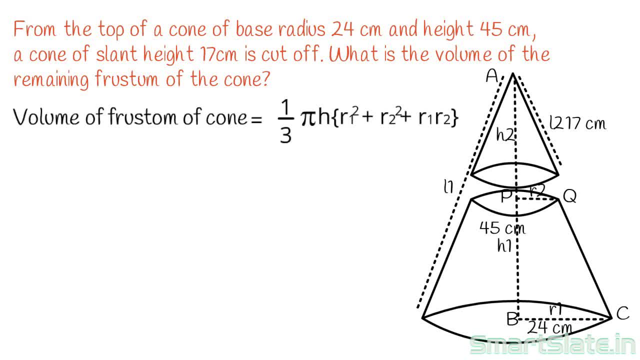 Volume of frustum of cone can be found using the formula 1 by 3 into pi, into h, in the bracket R1 square plus R2, square plus R1 into R2.. Notice, we don't have height of frustum of cone and radius of upper circle. Our first goal is to find the value of the. 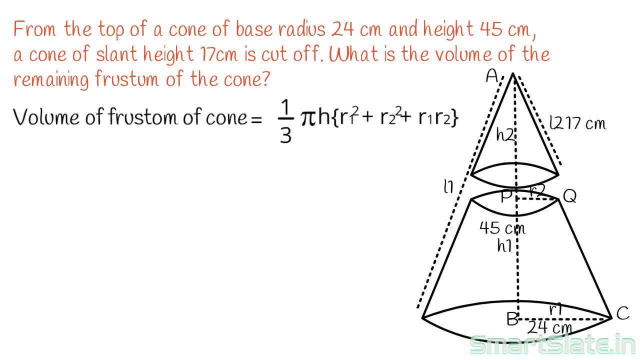 value of these items. Observe this figure. I have drawn the cone with cut off portion and frustum of cone. Let's call radius height and slant height of cone as R1, H1 and L1.. We have value of R1 and H1.. 24 centimeters and 45 centimeters, But we don't have the. 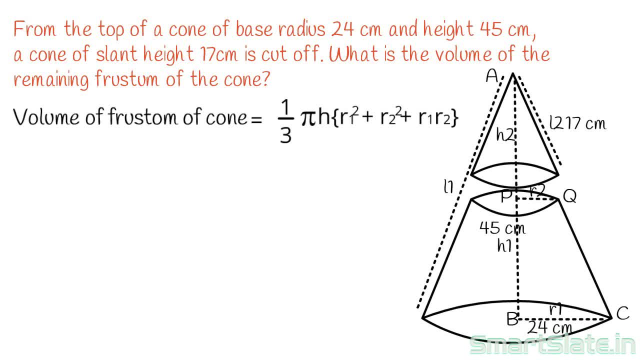 value of L1.. Slant height of cone: This is L2.. Slant height of the cut off cone. Value of L2 is 17 centimeters. The height of cut off cone be H2 and radius of upper circle is R2.. Observe the figure. 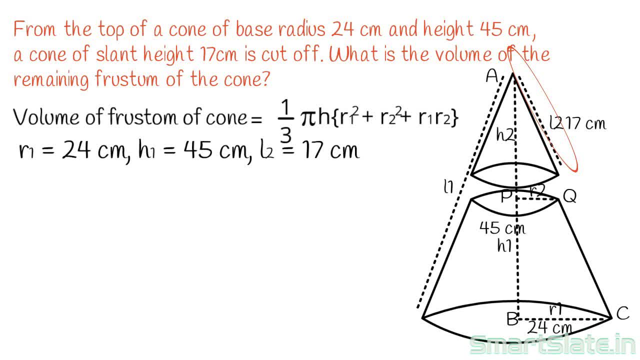 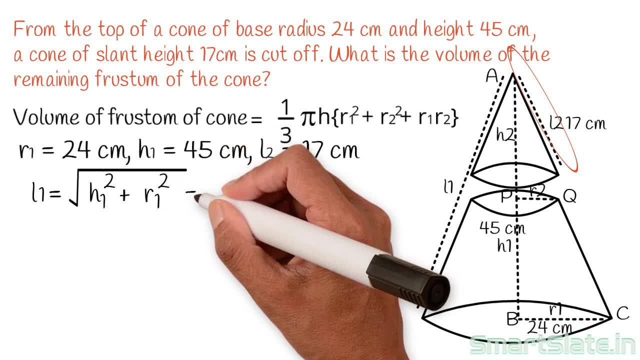 Using Pythagoras theorem, we can easily find the value of L1.. L1 is equal to square root of H1 square plus R1 square. It is square root of 45 square plus 24 square. 45 square is 2025.. 24 square is 576.. Hence, 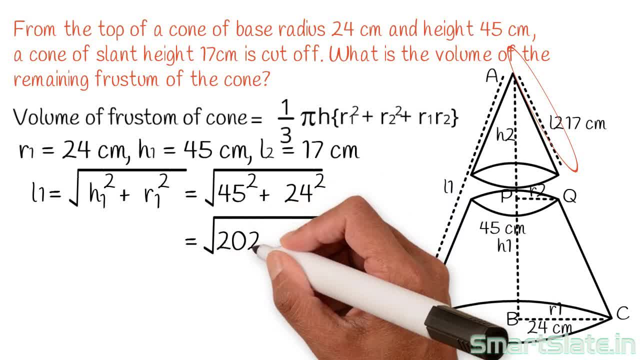 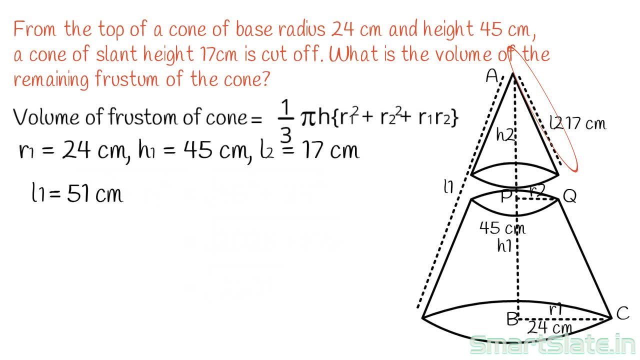 it is square root of 2025 plus 576.. It is square root of 2601.. Square root of 2601 is 51.. Hence, L1 is equal to 51 centimeters. If you look at the figure, the line of cut off is parallel to base. This makes triangle. 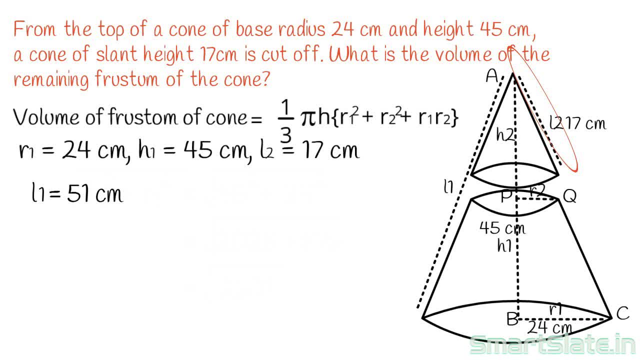 ABC and triangle APQ, similar triangles and hence corresponding sides are proportional. Hence R1 by R2 is equal to L1 by L2.. Except R2, we have all other values. It is 24 by R2 is equal to 51 by 17.. 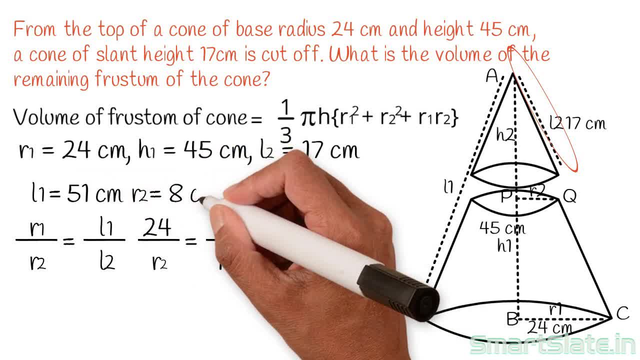 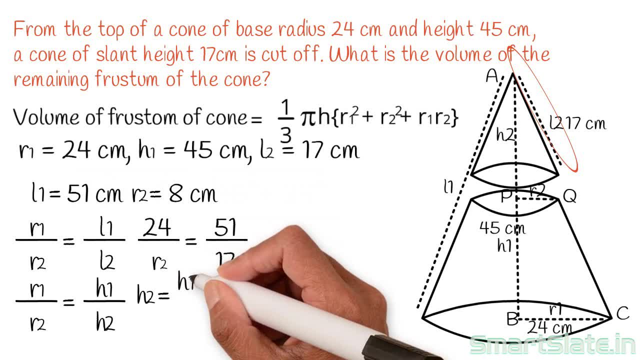 Hence R2 is equal to H1 by H2.. H2 is equal to H1 into R2 by R1.. Similarly, R1 by R2 is equal to H1 by H2.. H2 is equal to H1 into R2 by R1.. 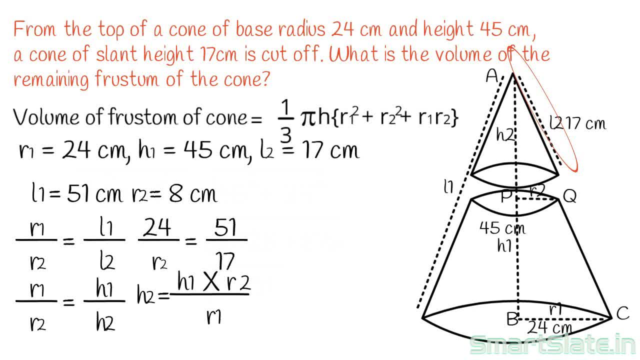 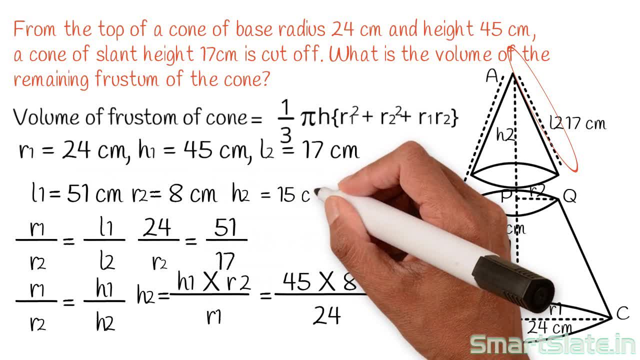 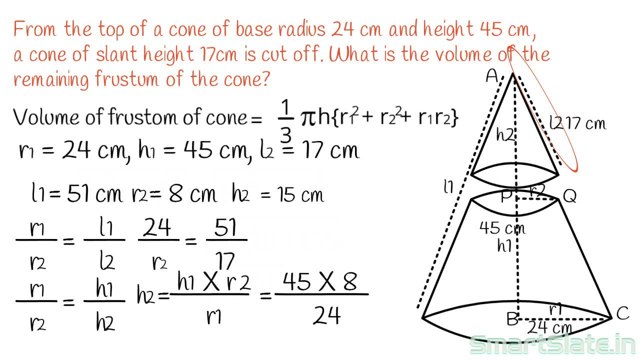 Substitute the values- H2 is equal to 45 into 8 by 24.. Hence H2 is equal to 15 centimeters. H2 is height of cut off cone. So height of the frustum of cone is different than the height of the first round of the. 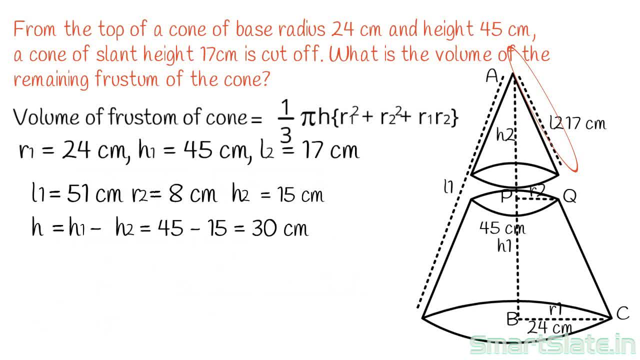 difference of height of entire cone and height of cut-off cone. Hence height of frustum of cone is 30 centimeters. Now we have values of height of frustum of cone and radius of upper circle as well. Now finding volume of frustum of cone is easy Formula to find. 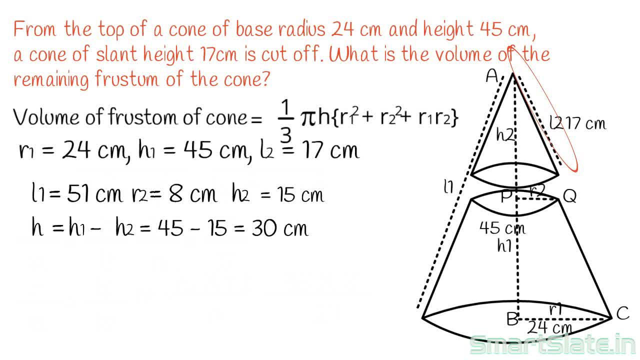 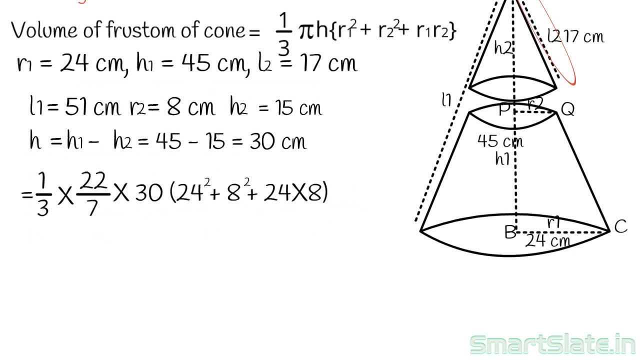 the volume of frustum of cone is 1 by 3 into pi into h, in the bracket r1 square plus r2, square plus r1 into r2.. Substitute the values of h, r1 and r2.. It is 1 by 3 into 22 by 7. 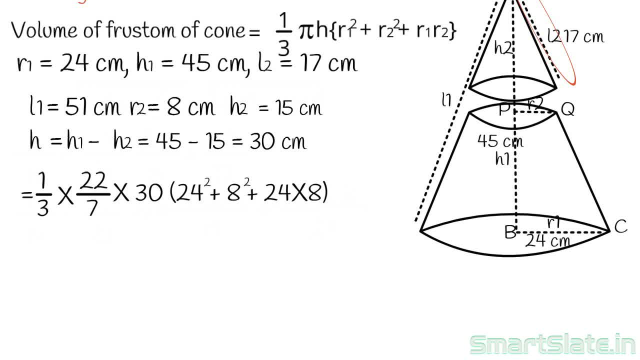 into 30 in the bracket 24 square plus 8 square plus 24 into 8.. 24 square is 576.. 8 square is 0.. 24 into 8 is 192.. Hence it is 22 by 7 into 10 in the bracket 576 plus 64 plus 192.. It.